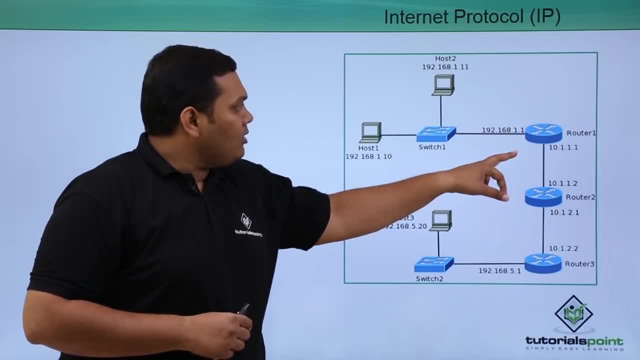 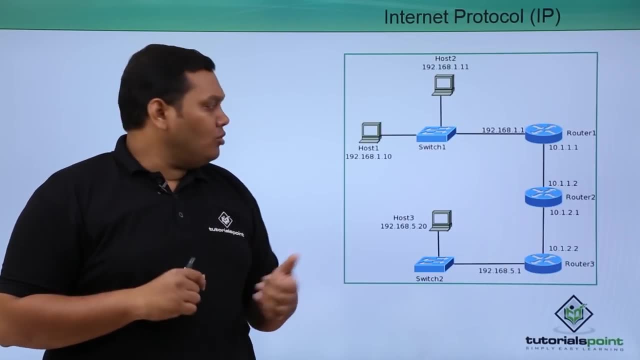 This is a separate network. So, двlarınė, this is a separate network and this is a separate network. and here when you switch from one router to other router, it is called as a hop and you can see IP addresses given to this host switch and routers also. 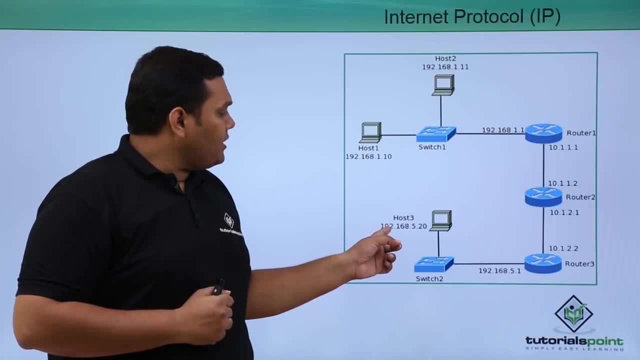 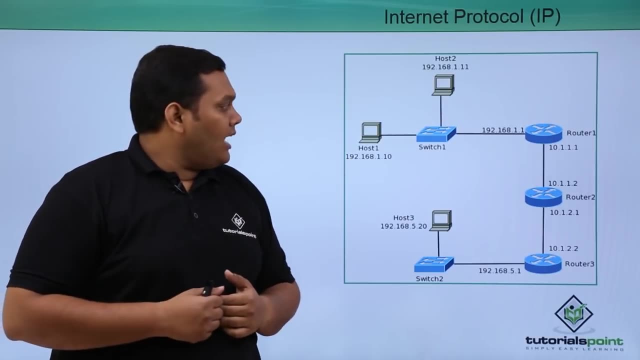 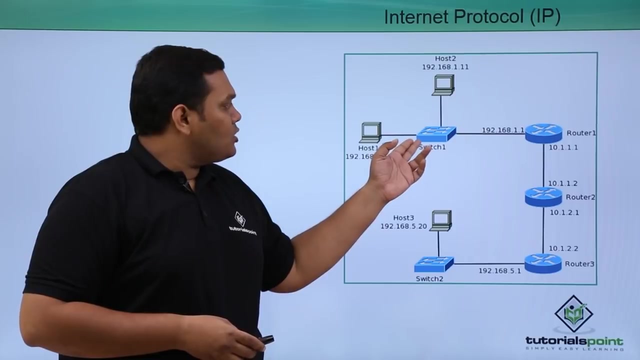 You can see, the host 3 consists of 192.168.5.20 IP address. in the same way, host 1 and host 2 are assigned with the IP address and routers also have the IP address based on the interface they are configured, and you can see switching of the networks. from this network, the data. 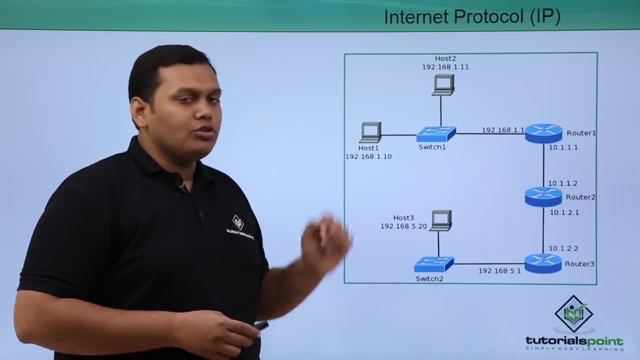 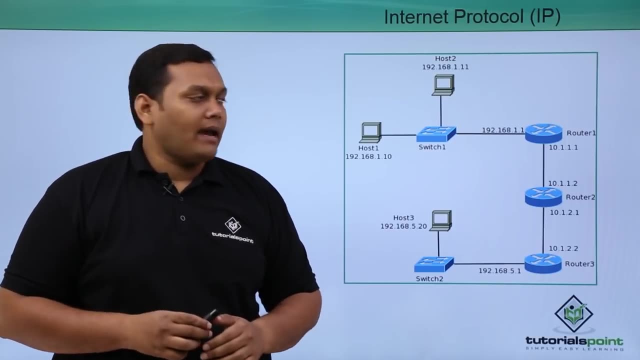 can be switched, or switch internet packeting can be happen to host 1 also. So this is the best example for the hop count, the IP addressing and also switching of the internet packeting. So you can see, considering the inter network, what we have discussed in the previous slide. 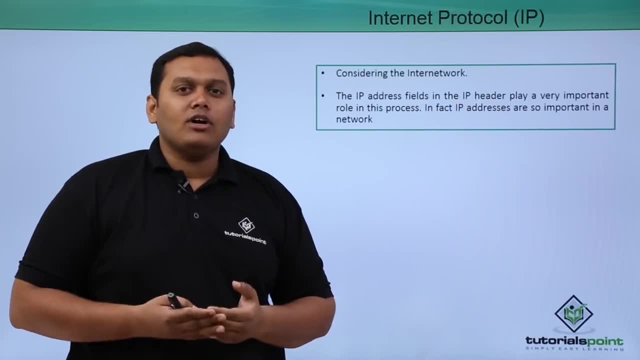 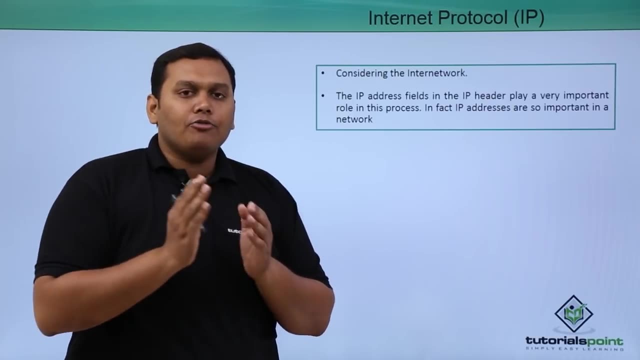 the IP address fields in the IP header play a very important or a key role here, So that the IP addresses are so important to transfer or transfer the IP address, Transmit the data from source to destination, and you can see here about the header of the 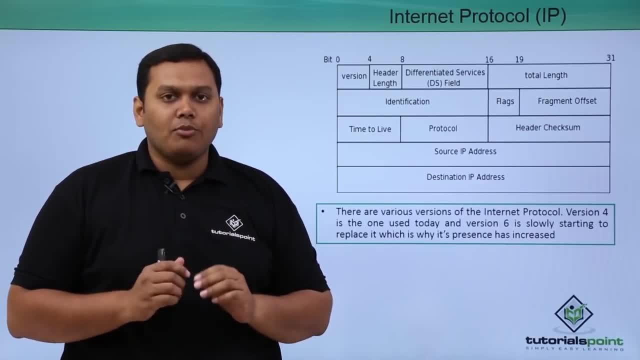 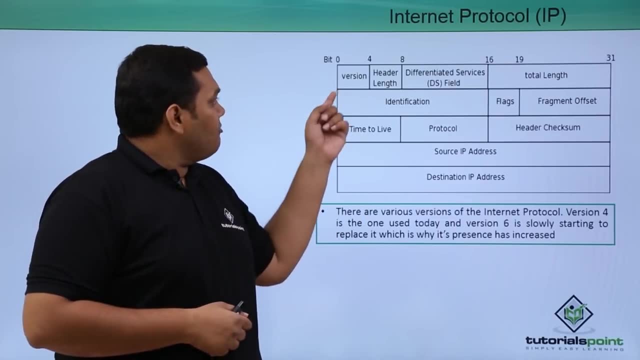 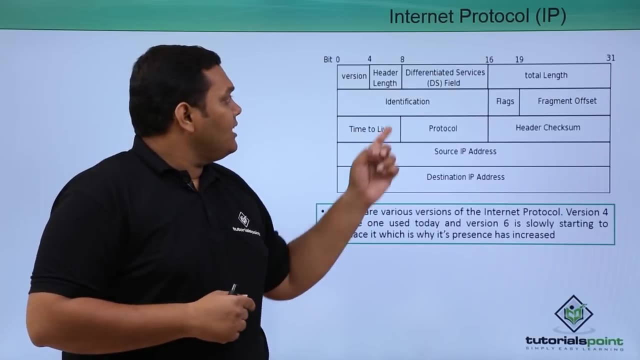 IP protocol. the internet protocol has a header, as we discussed about the source information and destination information, and in the header, the, it is segregated or segmented as version. which version is the IP we are using? and header length. what is the header length or what is its size? differentiated services field. 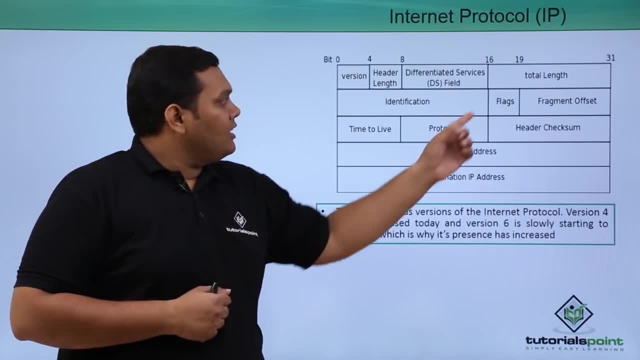 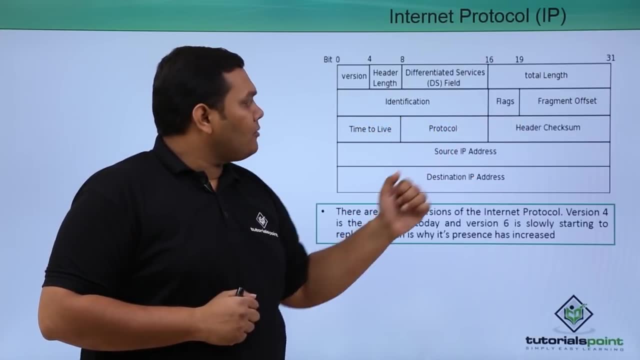 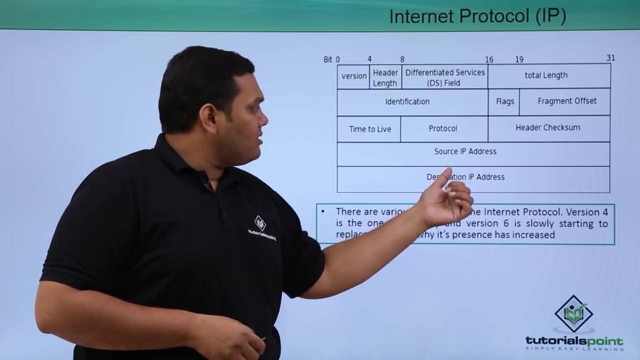 So what this field functions and what is the size of this field? Total length. total length of the information available in the header file: identification flags, fragment, offset, time to life, protocol and header checksum we will be discussing in the next slides. and also you can see about the source IP address and destination IP address. 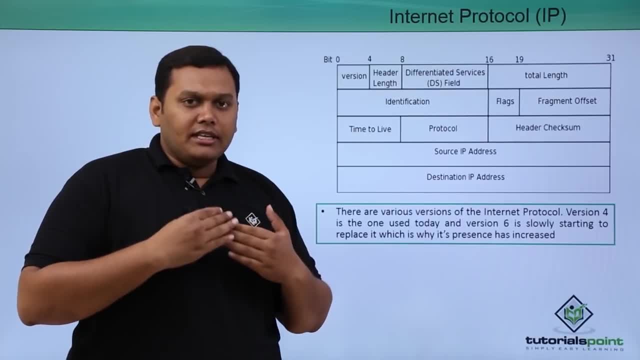 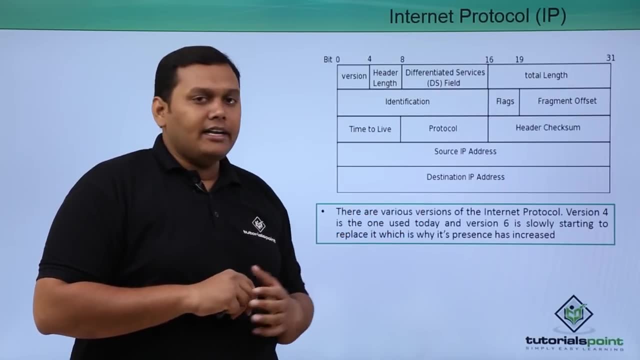 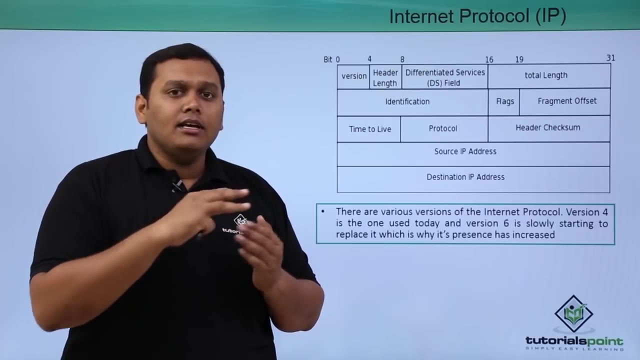 So what is source IP address? the data from which it is sent through the network is called a source, and the source IP address is information available in the header file So that it- the destination host, Host or the destination device- knows from where the data is been coming from and the 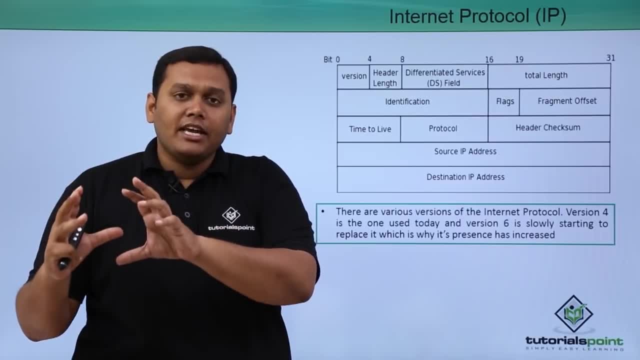 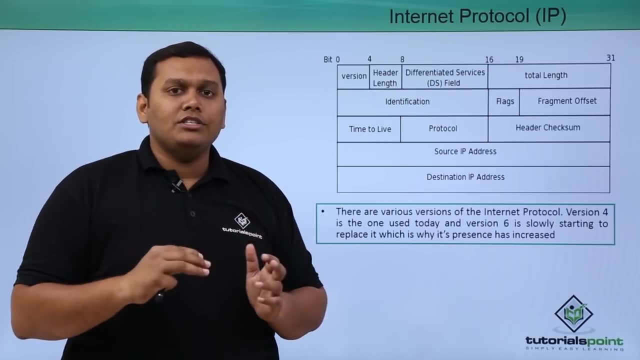 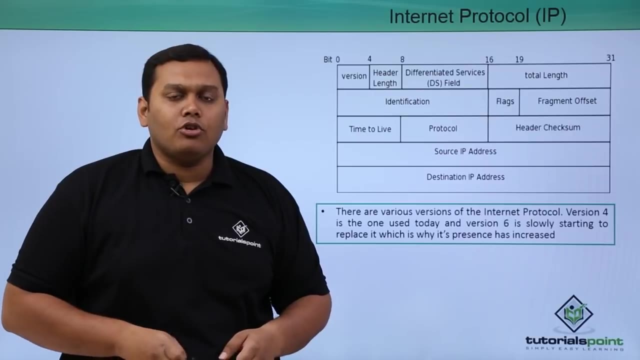 destination IP address is also present here, So that the destination IP address is informed, or the destination host is informed that some data is coming on your way, So it can acknowledge it by the acknowledgement. There are various versions of internet protocol. So there are various versions of internet protocol, but now presently version 4 is been 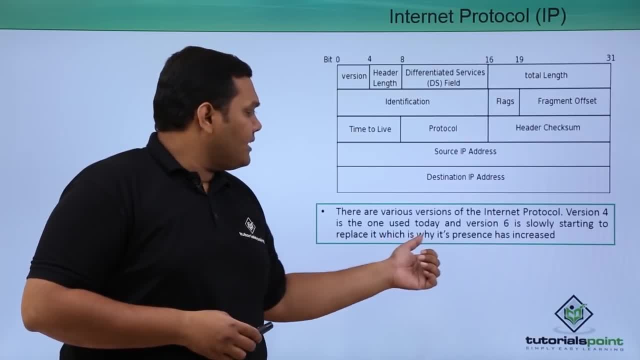 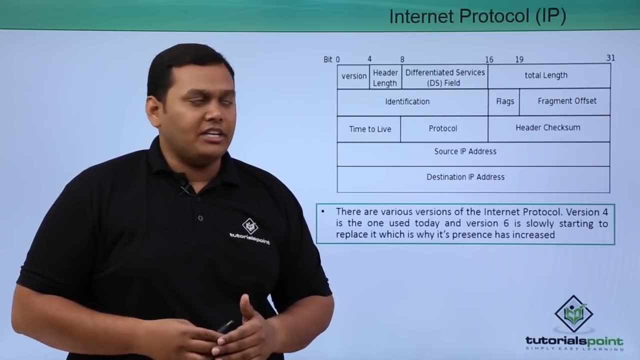 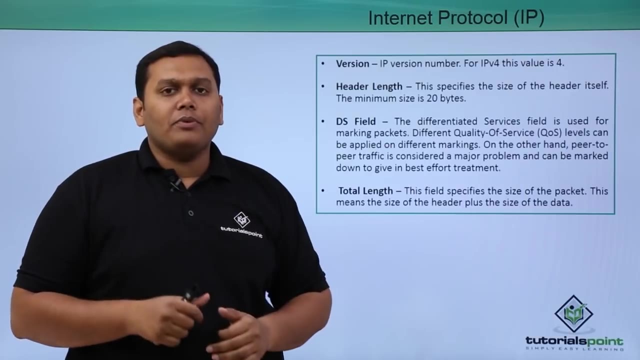 used today And version 6. It is getting its importance. in the next year or other year it can come into existence or full fledge of functioning here and you can see version. as I said, we will be discussing in the next slides in the header what each and every topic is discussed here. 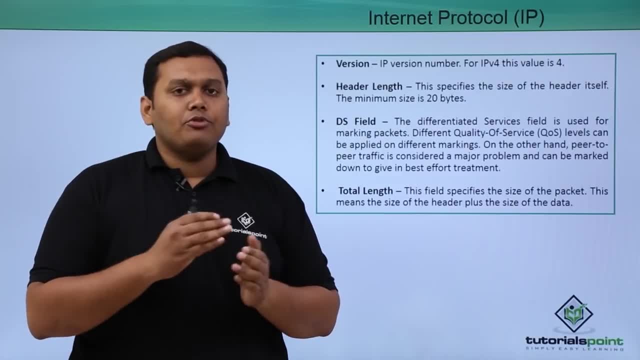 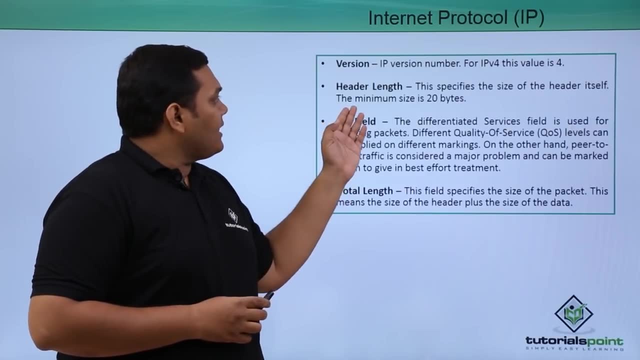 So version: IP version number. So what is the IP version internet protocol version which we are using presently? we are using IPv4 and this value is 4 in bits. header length: What is the header length? Header length is 20 bits in size or 20 bytes in size? this specifies the size of the header. 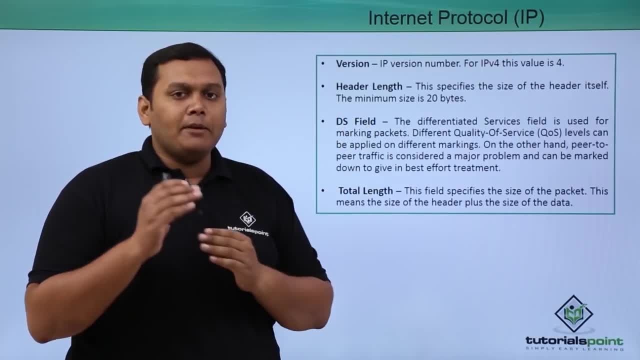 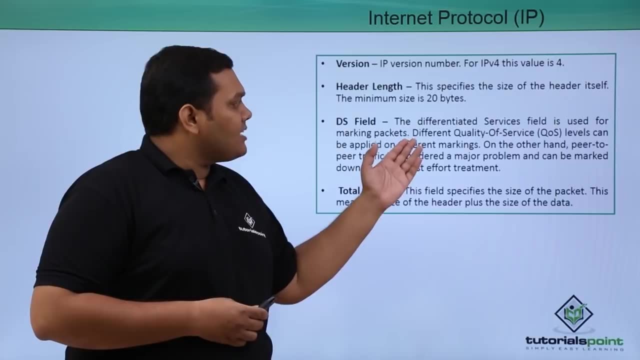 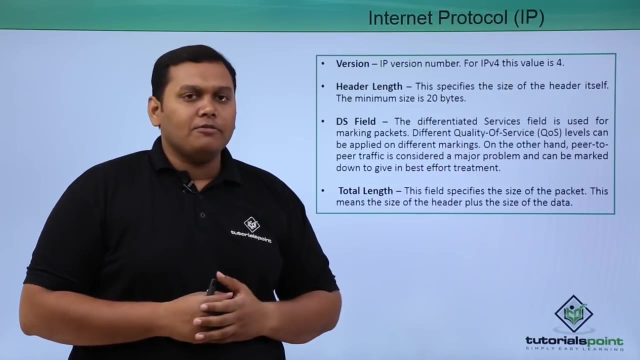 itself and also the minimum size is 20 bytes and it can be maximum of the depends on the header file size, DS field- as we discussed about the differentiated services field, it is used to mark packets. in the fragments I can see QoS, quality of service is also considered in this DS field and the different markings. 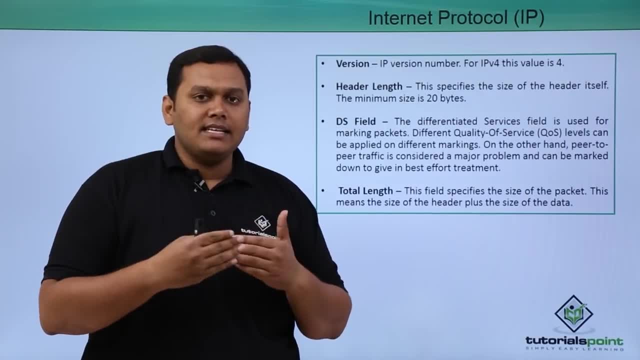 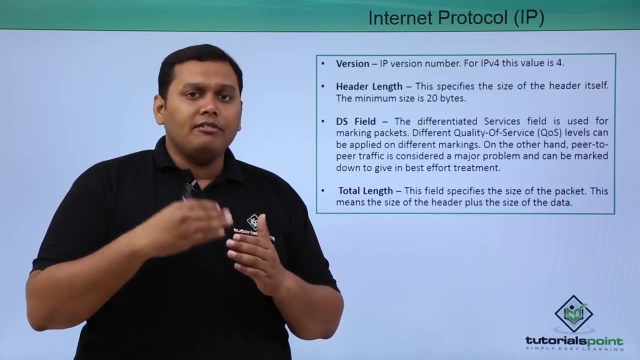 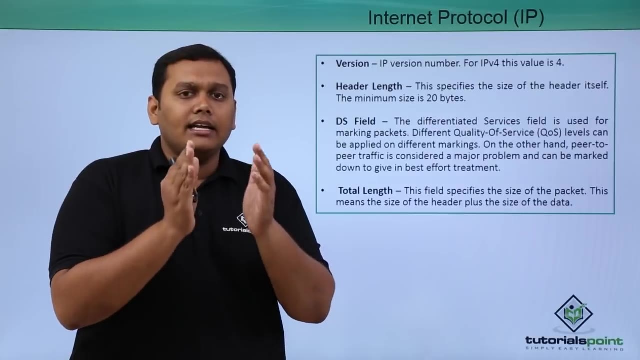 based on segments. As you know, TCP and UDP sends in the segments and here the segments are again fragmented in the fragments section and so that it can be given single markings for each and every fragment, so that a segment can be collided with the all fragments and it can be given some numbers here. and 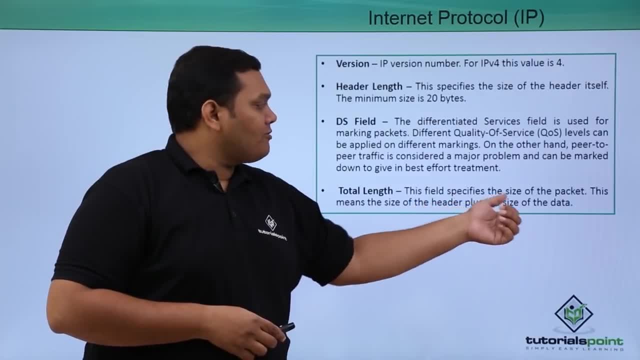 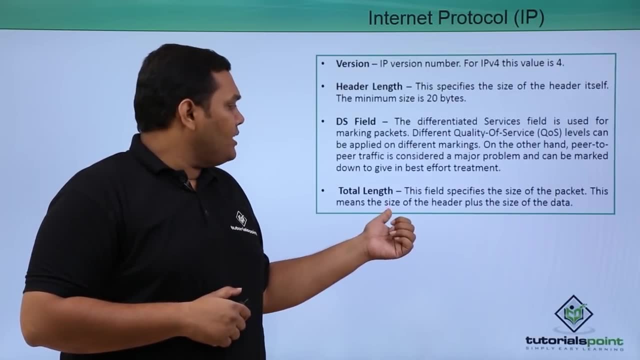 you can also see total length. This field specifies the size of the packet so you can see the total length. or the size of the packet is specified in the header file so that the mean, the size of the header plus in the size of the data, is available in the total length of the header file, so that all 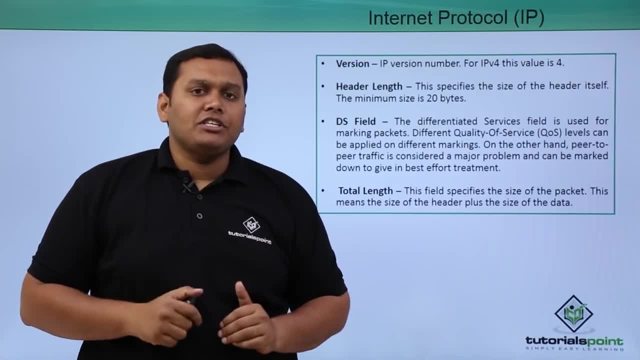 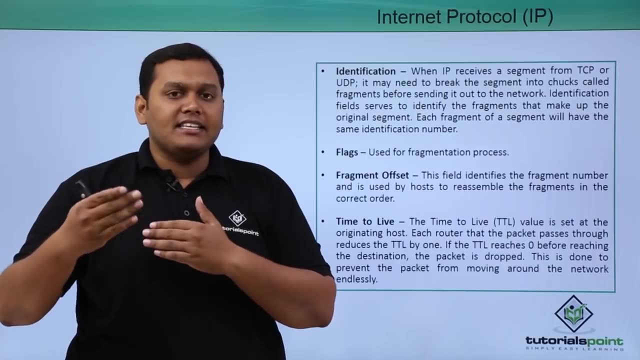 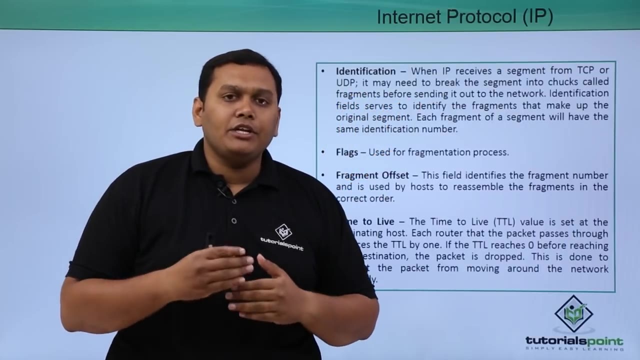 the version number. all the details are clearly mentioned in the header file about the total length of the header and you can see here identification how the IP identifies and receives information. when IP receives the segment from TCP or UDP, it may need to break the segment, as we discussed. it may need to break up in the form of chunks of about the segments and 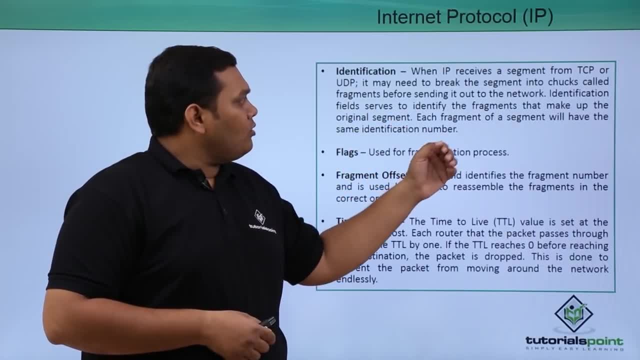 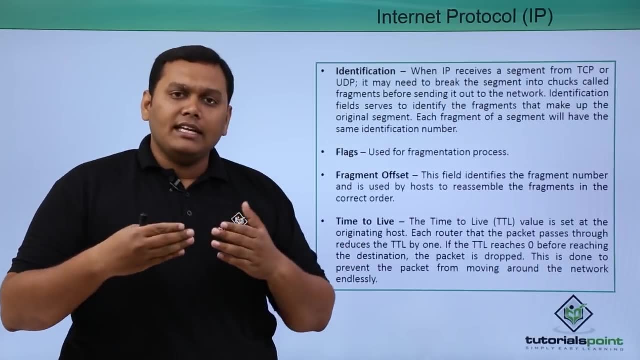 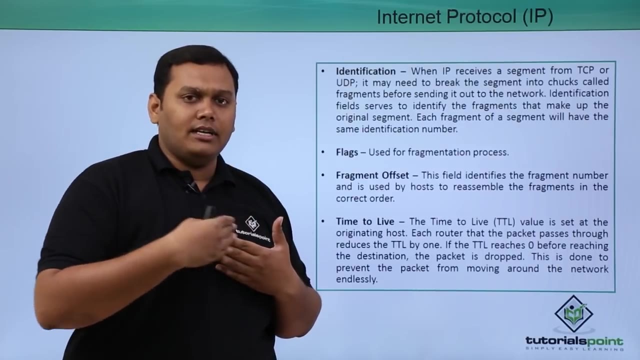 it is called as fragments here and before fragments are sending out, Fragments are sending out into the network. identification field serves this one and it gives identification to each and every fragment so that in a network, in a parallel path, many packets can be forwarded or many fragments can be forwarded simultaneously. 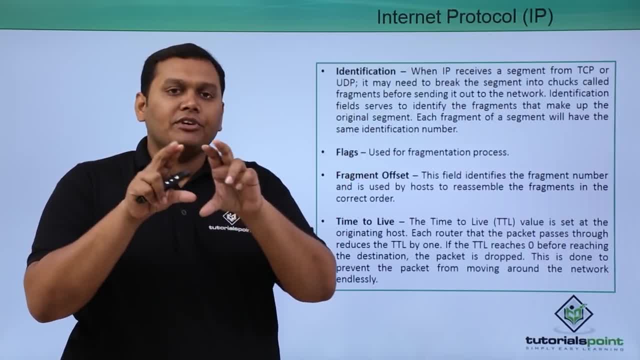 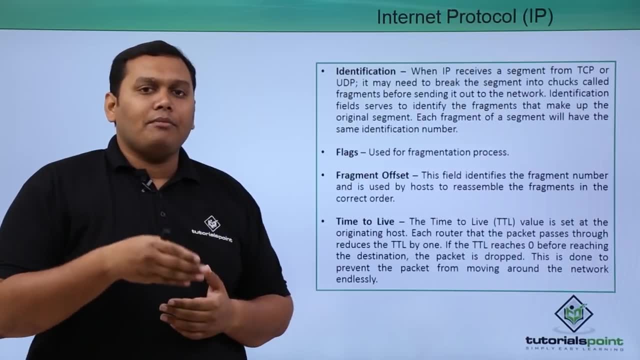 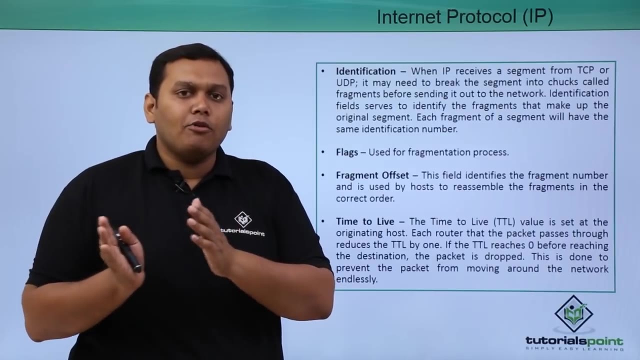 so that before, because of this marking field, it can have the information very clearly and it can collide after receiving to the destination and you can see flags using fragmentation process. so what is the fragmentation process? we have discussed in the identification, fragmenting each segment and giving it a separate field details so that it can be forwarded to the. 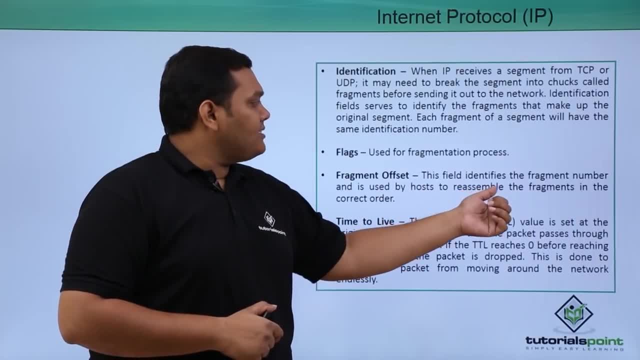 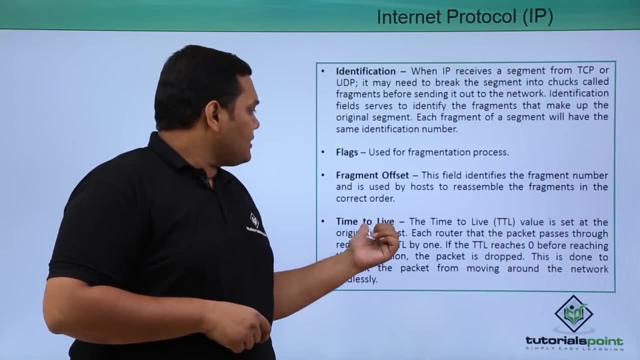 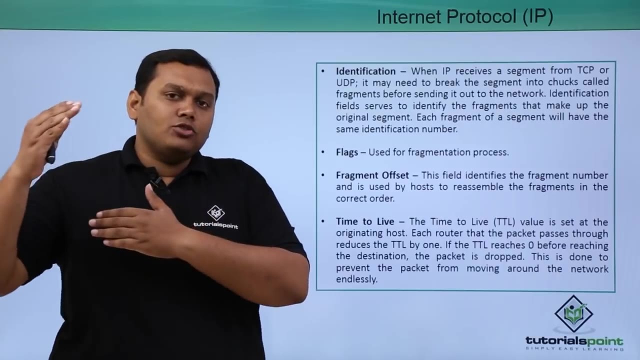 destination Fragment offset. this field defines the fragment number is used by host and resembles the fragment in the destination host. also, in the correct order time to live. the time to live or TTL value is set at the originating host. that means when the source is sending details. it. 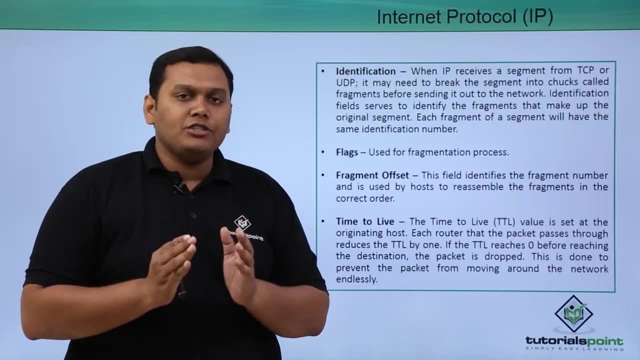 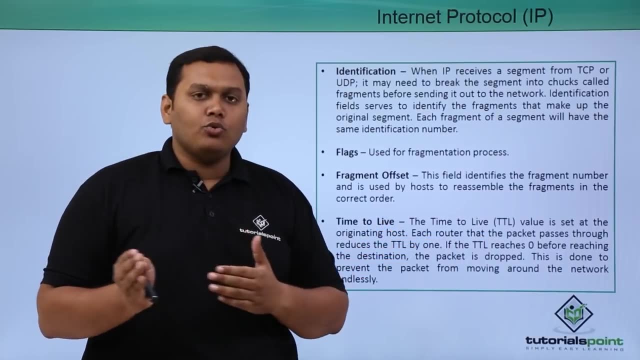 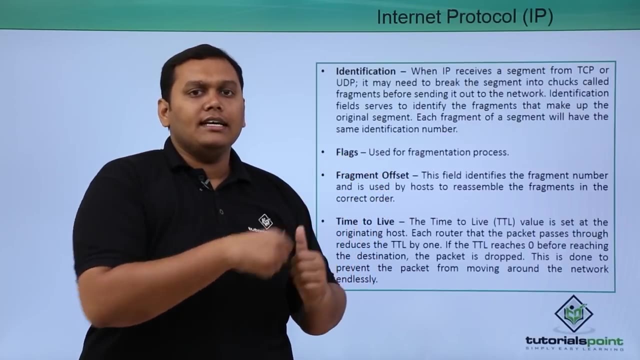 will have the TTL value also assigned to the packets or segments or fragments so that, based on the TTL value, the originating host, each router that packet passes through it, will have this value and passes this to the next level router or next level switch to switch it to the destination host. you can see about the protocol. what is the protocol as per the? 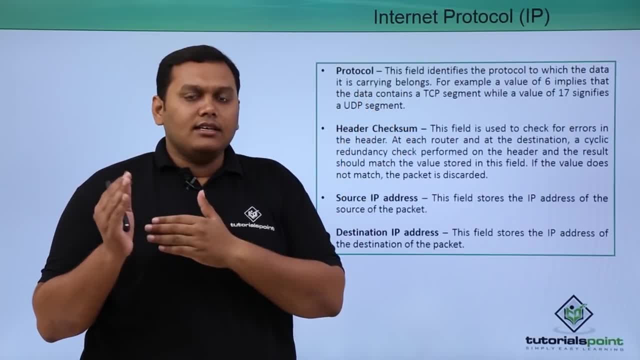 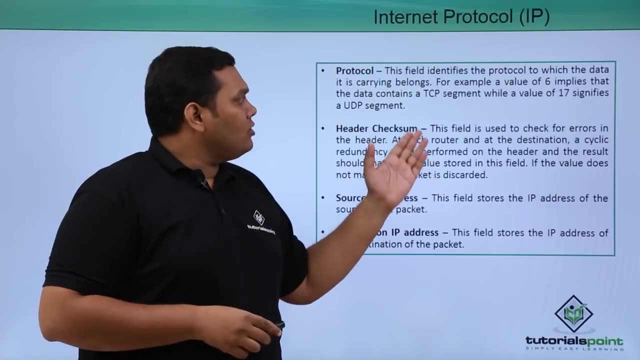 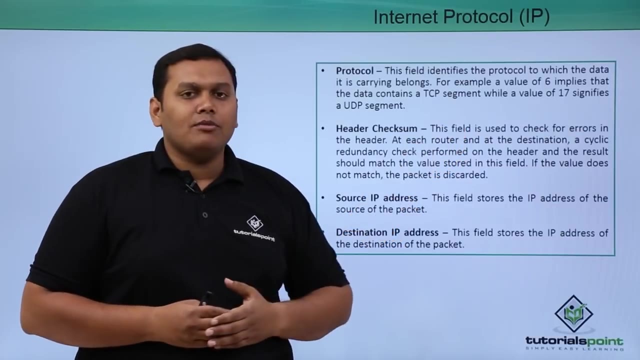 definition you can see the protocol the data carrying belongs to. has a separate IP address or given a separate header, clearly given as a address and also the value implies. for example, if you take So 6 implies the TCP information and here 17 signifies about the UDP information, about 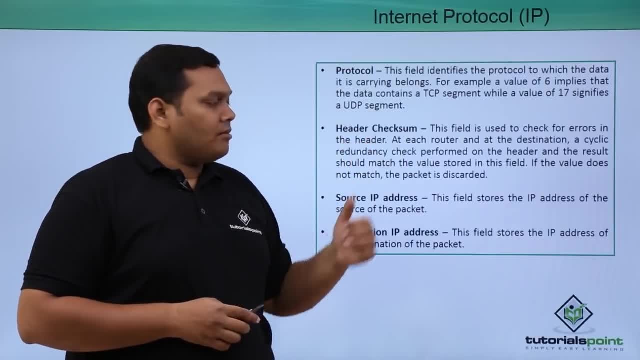 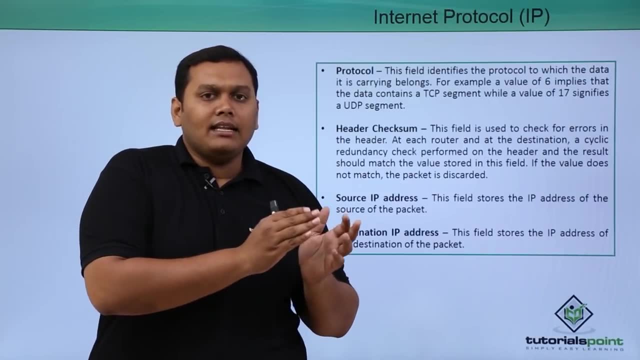 the segments we are speaking all about and you can see header checksum. and this is important to error handling: when a error occurs that take an example that a data is transferred to destination but we do not have an acknowledgement that is there is some error, so that this checksum 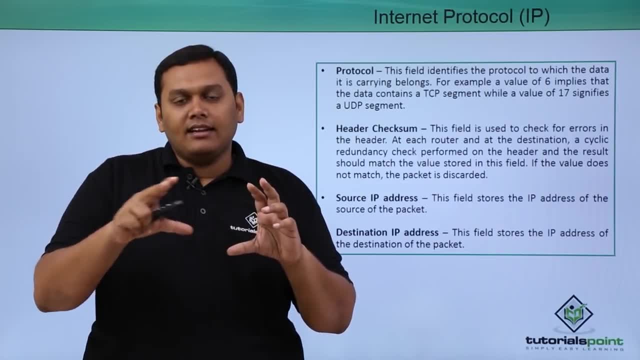 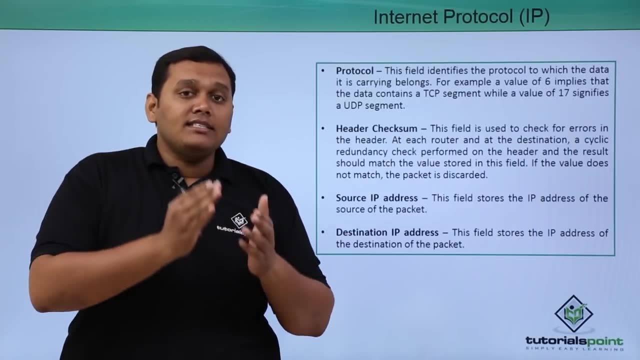 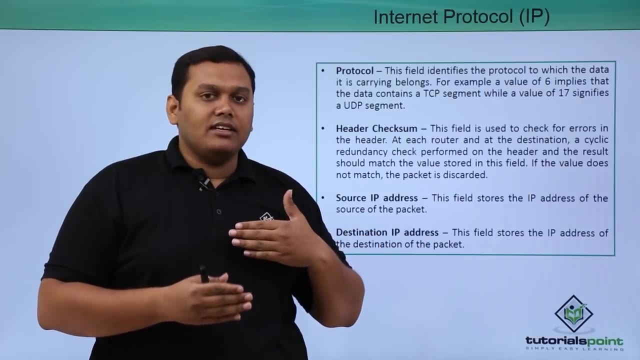 value is assigned to that header. so if there is an error the destination does not revert back again. it sends the same information Until the destination acknowledge the information about the data received to it and source IP address and destination IP address. as you know, source IP address is important here, so 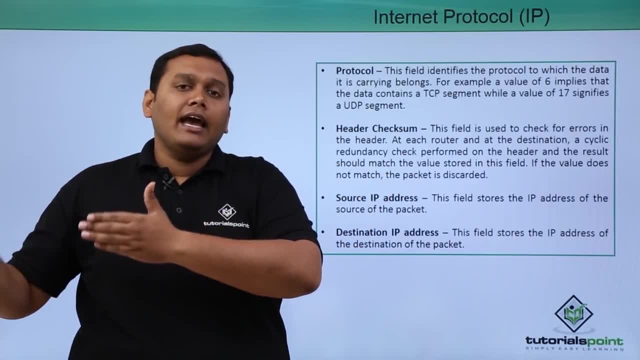 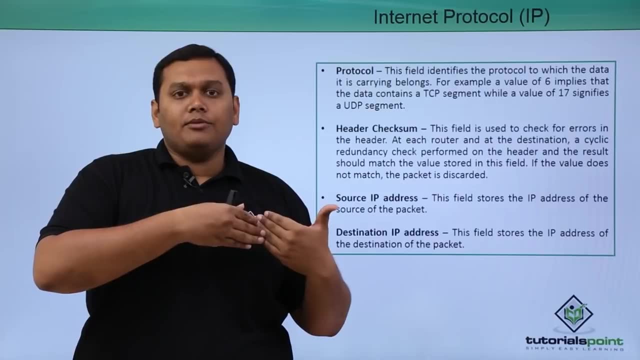 that from where the data is coming the destination will be acknowledging and also about the destination IP address. the source should be knowing about the destination IP address so that it can get acknowledgement from the destination and it can know that the data has been transferred to the destination host and it is important.